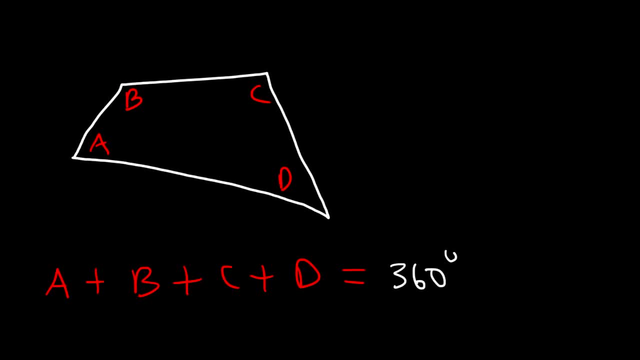 angle D adds up to 360 degrees. Now there are certain types of quadrilaterals that have specific names. This particular quadrilateral is the trapezoid. In this figure, these two lines are parallel. Now, if you have an isosceles trapezoid, 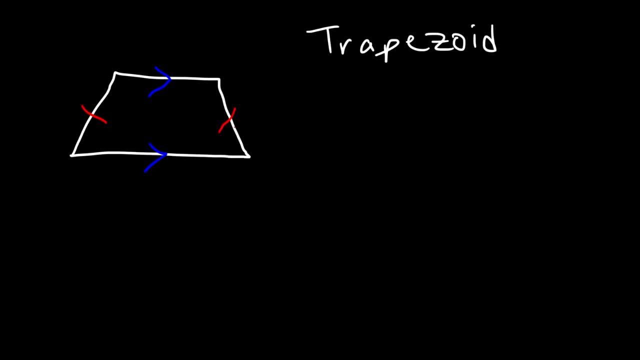 these two sides are congruent, so make sure you're aware of that. In addition, the angles opposite to those two sides are congruent. if it's an isosceles trapezoid, The next shape that you need to be familiar with is the. 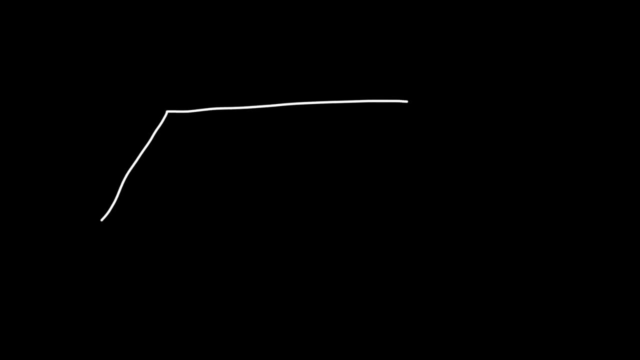 parallelogram, which looks like this: In the parallelogram, these two lines are parallel, and these two lines are also parallel. In addition to being parallel, the opposite sides are congruent. so those sides are congruent and these two sides are congruent as well. So that's the parallelogram. Keyword: parallel: 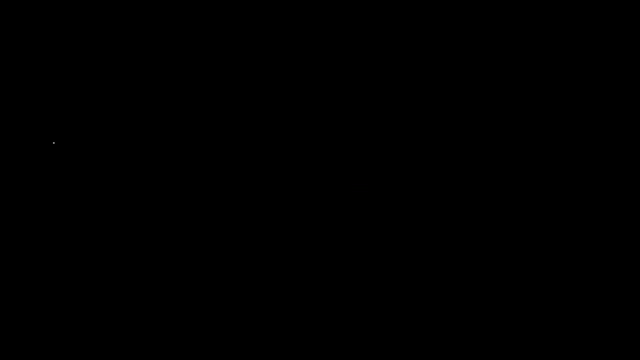 Opposite sides are parallel to each other. The next figure that you need to know is the rectangle. In the rectangle, all four angles are congruent. They're all right angles: 90 degrees 90 times 4 is 360.. Opposite sides. 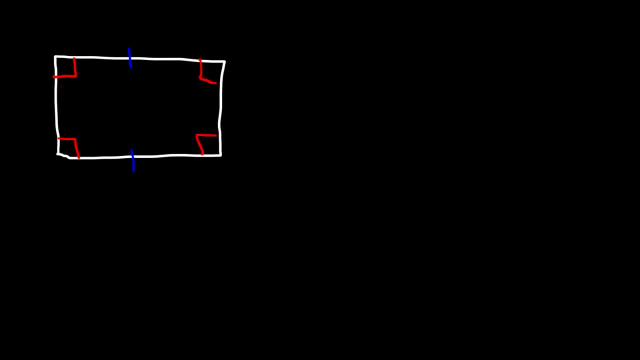 are congruent. these two sides are equal to each other and the opposite sides are parallel as well, so the rectangle is like a parallelogram, but the angles are 90, so these two sides are parallel to each other and the top and bottom line are: 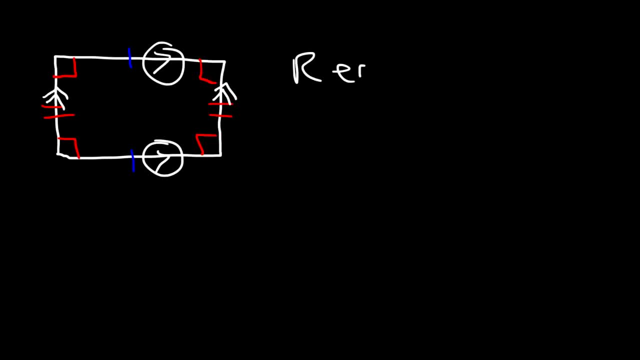 parallel to each other. so that's the rectangle. the next shape that you need to be familiar with is the rhombus. in the rhombus, all four sides are congruent to each other. this might not be drawn to scale, but it's supposed to be like that. let me draw a better picture. 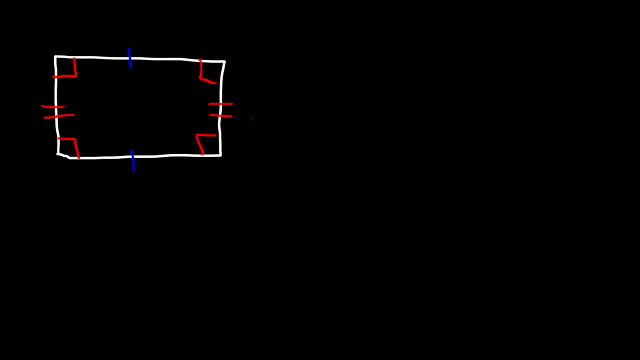 these two sides are equal to each other and the opposite sides are parallel as well, so the rectangle is like a parallelogram, but the angles are 90, so these two sides are parallel to each other and the top and bottom line are parallel to each other. so that's the rectangle, the next shape that you need. 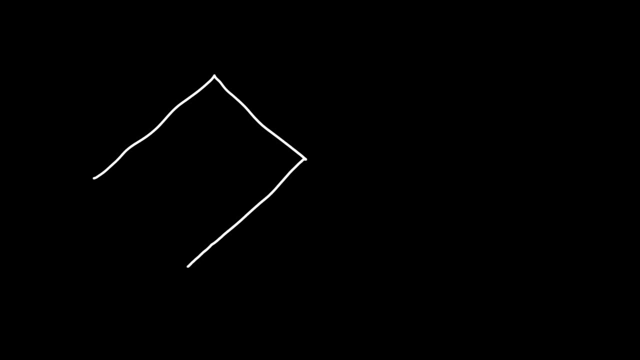 to be familiar with is the rhombus. in the Rhombus, all four sides are congruent to each other. this might not be drawn to scale, but it's supposed to be like that. let me draw a better picture. so all four sides are congruent and the diagonals 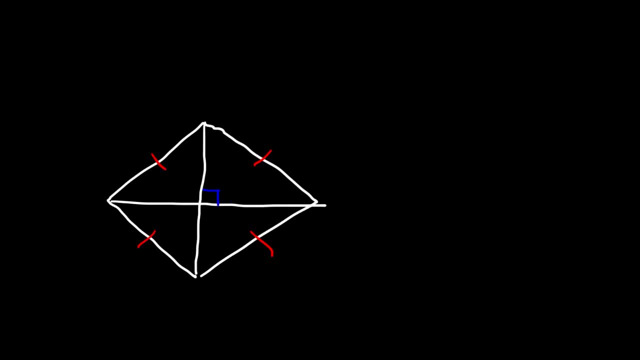 bisect each other at right angles, So each of these angles are right angles. The square is similar to a rhombus and a rectangle, but also different from each. Like a rectangle, all four angles of a square are 90 degrees and like a rhombus, 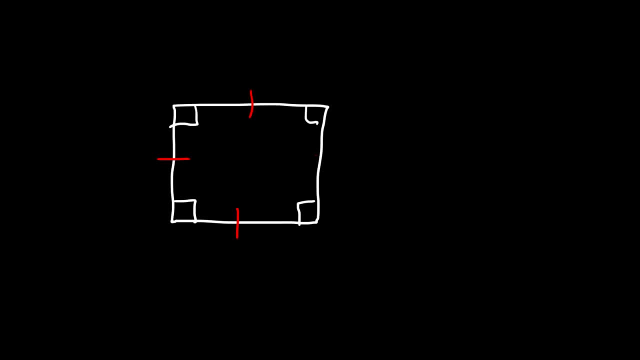 all four sides are congruent. So in a square, everything is basically equal to each other And, like a parallelogram, opposite sides are parallel to each other, So each of these shapes are known as quadrilaterals. Now let's work on some. 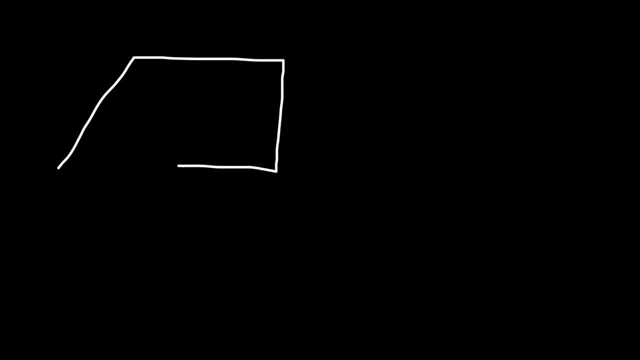 math problems. So let's say, if we have this four-sided quadrilateral, Let's say this is X and this angle is X, It's 58 degrees and this one is 73 and this angle is 117 degrees. Go ahead and find the value of X. Now, if you recall the sum of all the interior angles of a. 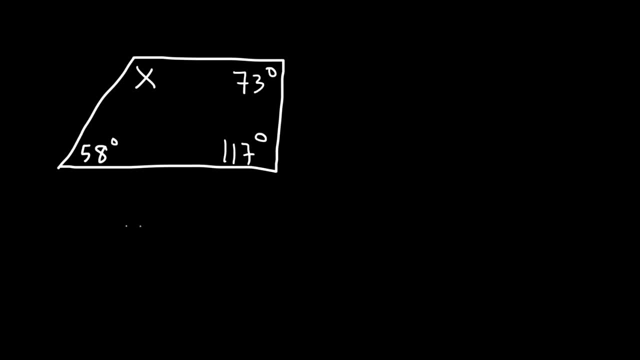 quadrilateral, a four-sided figure adds up to 360. So that means 58 plus 73 plus 117 plus X. All four angles have to add up to 360. If we add 58 and 73, that's 131.. 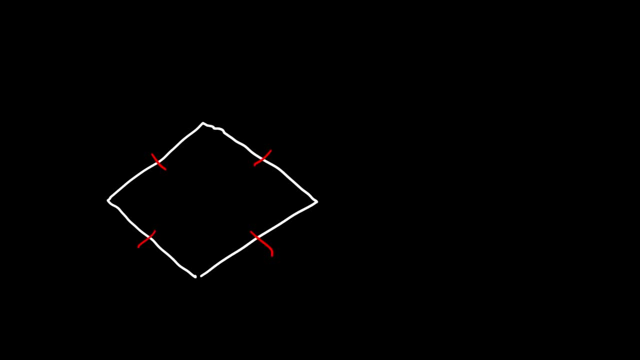 so all four sides are congruent and the diagonals bisect each other at right angles, so each of these angles are right angles. the square is similar to a rhombus and a rectangle, but also different from each. like a rectangle, all four angles of a square are 90 degrees, and like a rhombus, 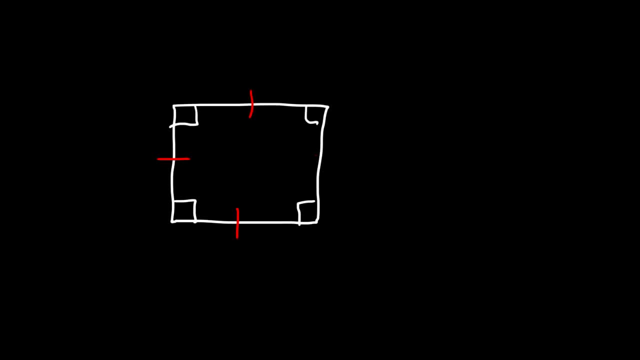 all four sides are congruent. so in a square everything is basically equal to each other and, like a parallelogram, opposite sides are parallel to each other. so each of these shapes are known as quadrilaterals. now let's work on some math problems. so let's say: if we have this four-sided quadrilateral, let's say: 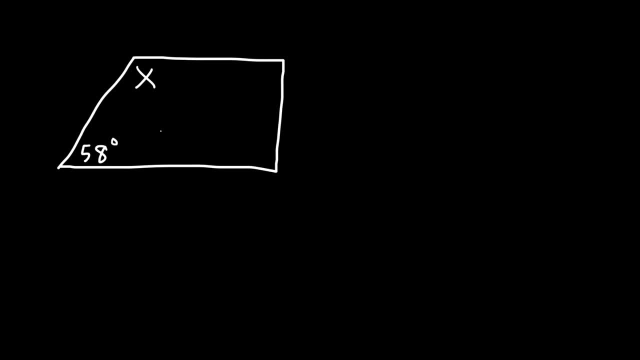 this is X and this angle is 58 degrees, and this one is seven 173 and this angle is 117 degrees. Go ahead and find the value of X. Now. if you recall, The sum of all the interior angles of a quadrilateral or four-sided figure adds up to 360. 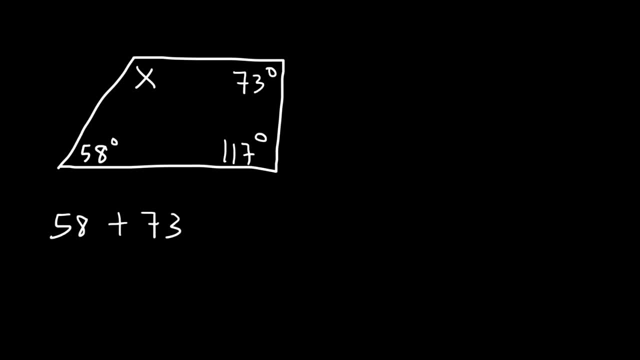 So that means 58 plus 73 Plus 117 plus X. all four angles have to add up to 360. If we add 58 and 73, that's 131. Next, if we add 131 plus 117, That's 248. so 248 plus X is equal to 360. 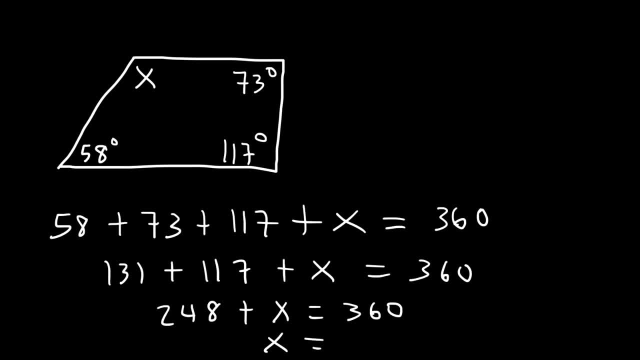 To find the value of X we need to subtract both sides by 248, so 360 minus 248 That's about 112. So that's how you could find the missing angle in a quadrilateral, As long as you keep in mind that all four angles have to add up to 360. 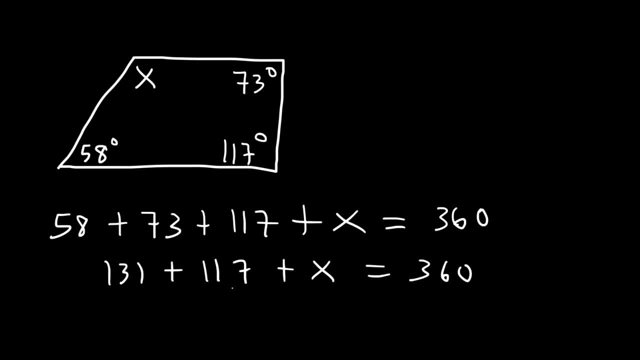 Next, if we add 131 plus 117, that's 248.. So 248 plus X is equal to 360.. To find the value of X, we need to subtract both sides by 248.. So 360 minus 248, that's. 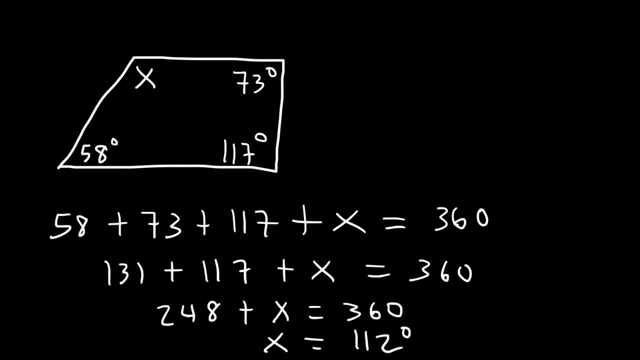 about 112.. So that's how you could find the missing angle in a quadrilateral. As long as you keep in mind that all four angles have to add up to 360,, it's going to be a piece of cake to solve these types of problems. 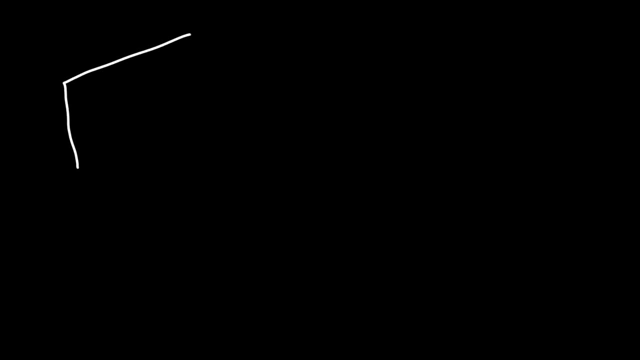 Now let's work on another example. Let's call this angle A, B, C and D. So angle A is equal to 5 X plus 10.. angle B is 10x minus 30, angle C is 95 degrees and angle D is 4x. Go ahead and. 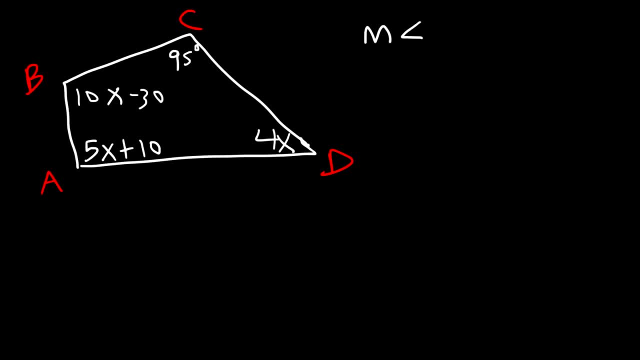 find the measure of angle A. Feel free to pause the video and work on this example. So we know that all four angles- A plus B, plus C plus D- has to add up to 360.. Angle A is 5x plus 10.. Angle B is 10x minus 30.. Angle C is 95.. Angle D is 4x. All of that. 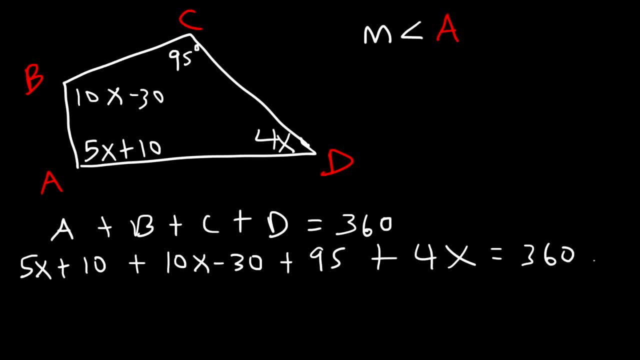 has to add up to 360.. So what we need to do is combine like terms: 5x plus 10x is 15x. 15x plus 4x, that's 19x. Negative 30 plus 95, or 95 minus 30,, that's 65.. 65 plus 10. 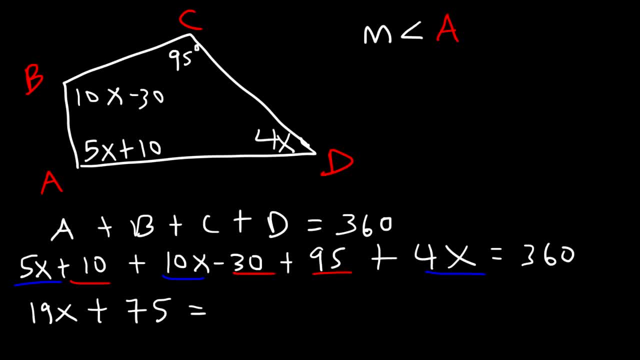 is 75.. So 19x plus 75 is equal to 360.. Now let's subtract both sides by 75.. 360 minus 75 is 75.. Now let's subtract both sides by 75.. 360 minus 75 is 75.. 360 minus 75 is. 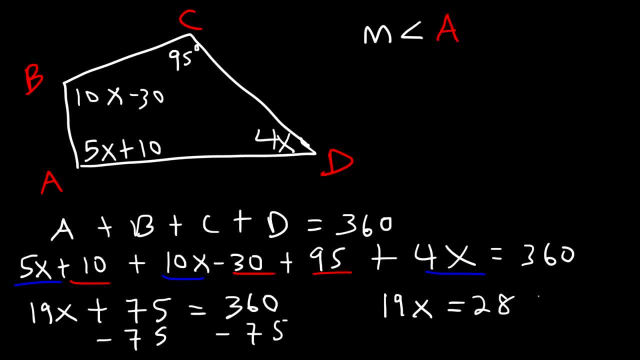 equal to 360.. Now let's subtract both sides by 75.. 360 minus 75 is equal to 360.. 360 minus 75 is equal to 360.. 360 minus 75 is equal to 285.. And 285 divided by 19 will give us: 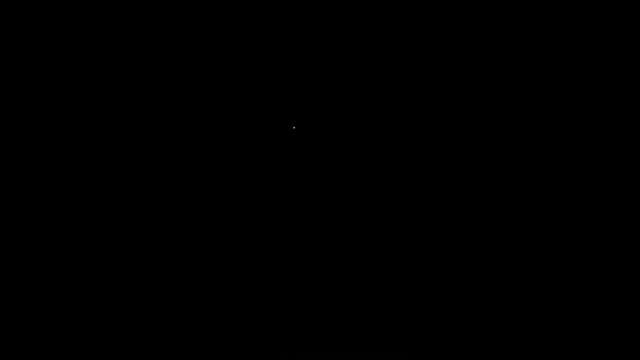 It's going to be a piece of cake to solve these types of problems. Now let's work on another example. Let's call this angle a, B, C and D. So angle a is equal to 5 X plus 10, Angle B is 10x minus 30.. Angle C is 95 degrees and angle D is 4x. Go ahead and find the. 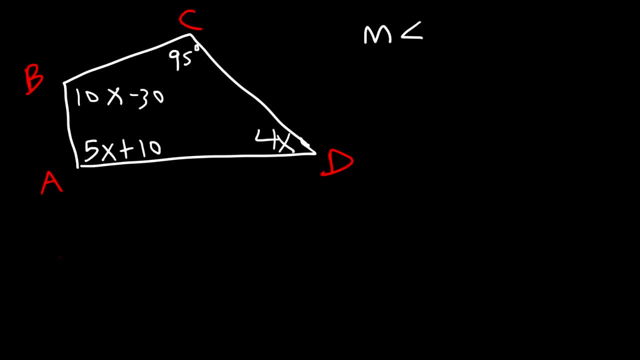 measure of angle A. Feel free to pause the video and work on this example. So we know that all four angles, A plus B plus C plus D, has to add up to 360.. Angle A is 5x plus 10.. Angle B is 10x minus 30.. Angle C is 95.. Angle D is 4x. All of that has to. 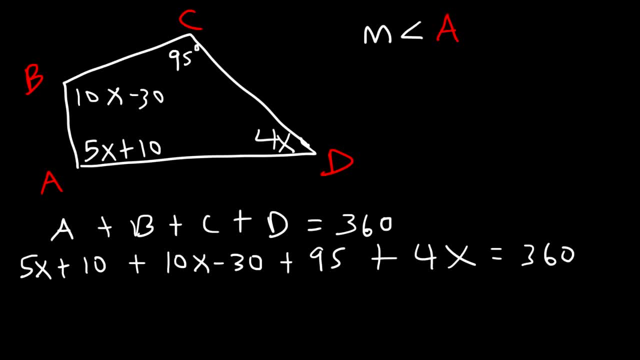 add up to 360.. So what we need to do is combine like terms: 5x plus 10x is 15x. 15x plus 4x, that's 4x, That's 19x. Negative: 30 plus 95, or 95 minus 30,, that's 65.. 65 plus 10 is 75. So 19x plus. 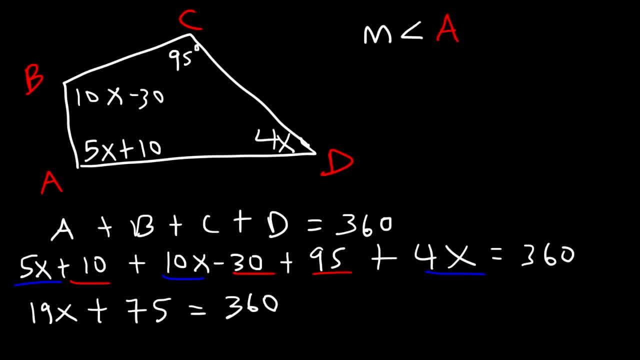 75 is equal to 360.. Now let's subtract both sides by 75.. 360 minus 75 is 285.. And 285 divided by 19 will give us an x value of 15.. So now that we have the value of x, 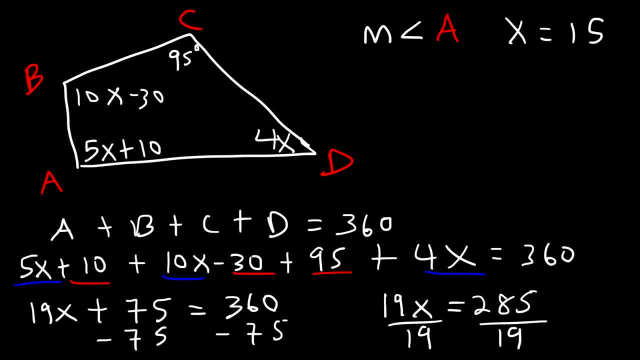 we can find any angle that we want to find. So let's go ahead and find angle A. So angle A is 5x plus 10.. And let's replace x with 15.. So it's 5 times 15 plus 10.. 5 times 15. 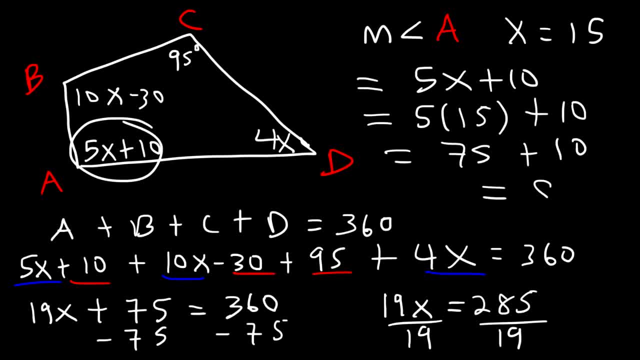 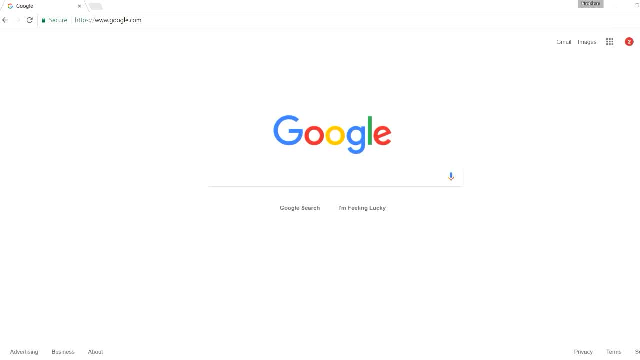 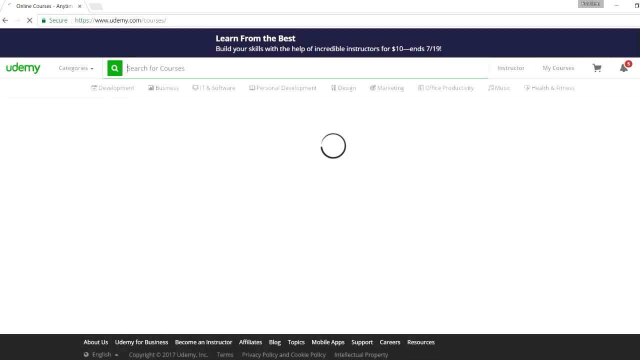 is 75.. 75 plus 10 is 85. So that's the final answer. It's 85 degrees. That's the measure of angle A. Now I want to show you one of my algebra courses that might be useful to you if you ever need it. So go to udemycom Now in the search box. 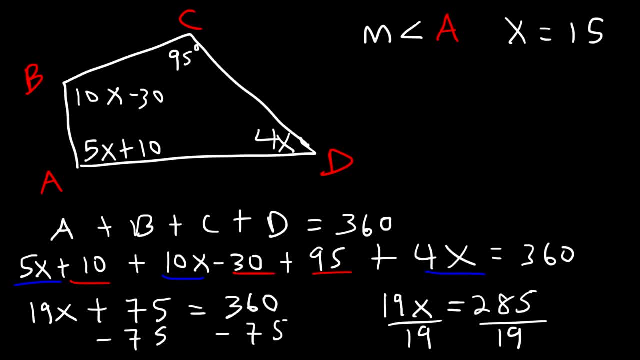 an x-value of 15.. So now that we have the value of x, we can find any angle that we want to find. So let's go ahead and find angle A. So angle A is 5x plus 10. And let's. 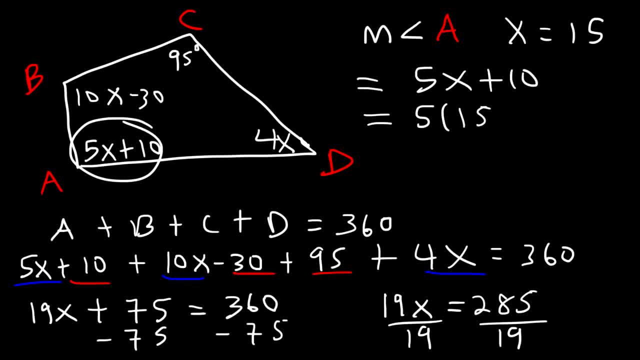 replace x with 15.. So it's 5 times 15 plus 10.. So angle A is 5x plus 10, and let's replace x with 15.. So it's 5 times 15 plus 10.. 10.. 5 times 15 is 75.. 75 plus 10 is 85.. So that's the final answer. It's 85 degrees. 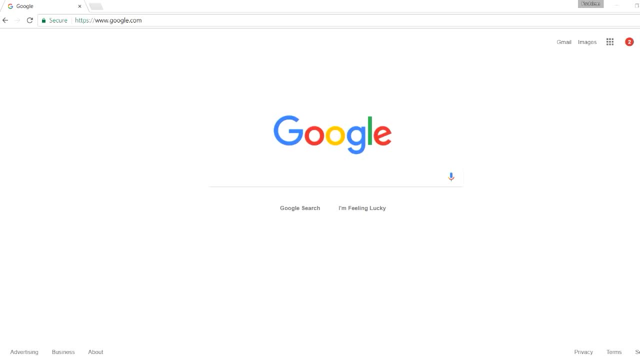 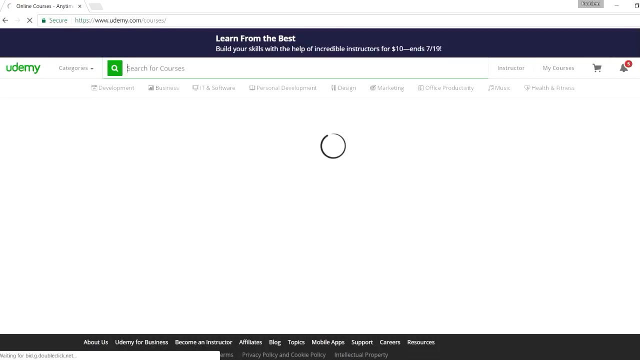 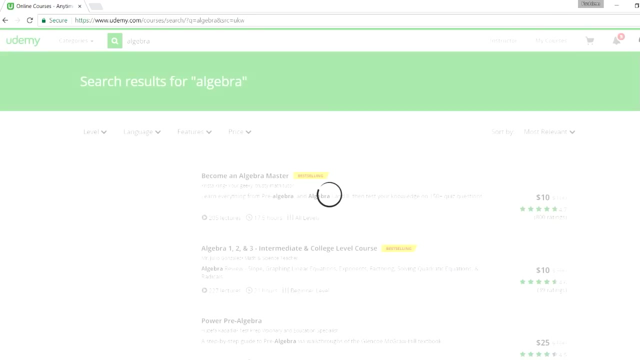 That's the measure of angle A. Now I want to show you one of my algebra courses that might be useful to you if you ever need it. So go to udemycom Now in the search box just type in algebra and it should come up. So it's the one with. 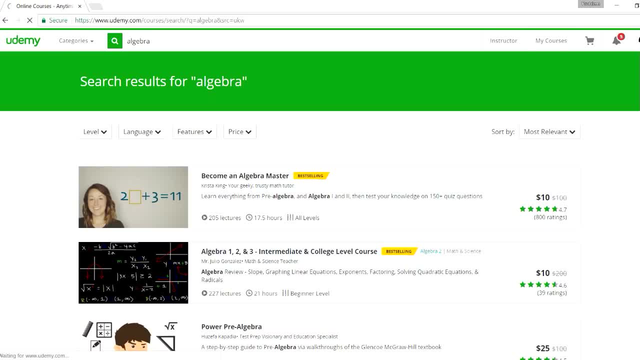 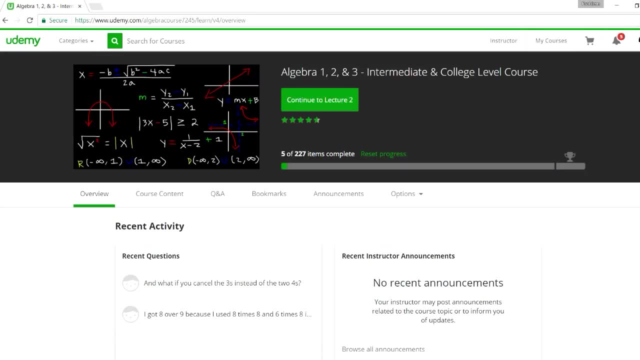 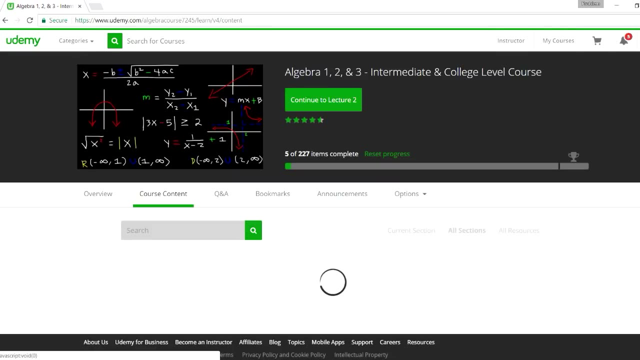 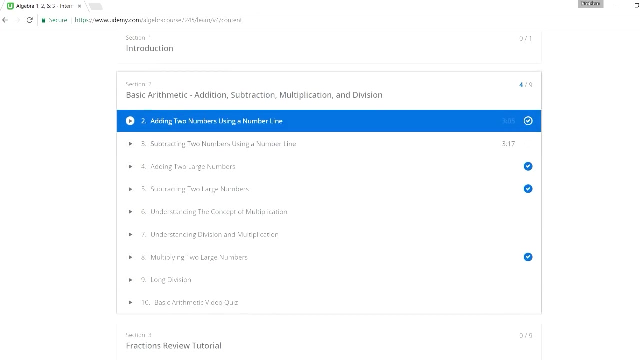 the image with the black background. So if you select that option and if you decide to go to Udemycom course content, you can see what's in this particular course. So the first section, basic arithmetic. for those of you who want to focus on addition, subtraction: 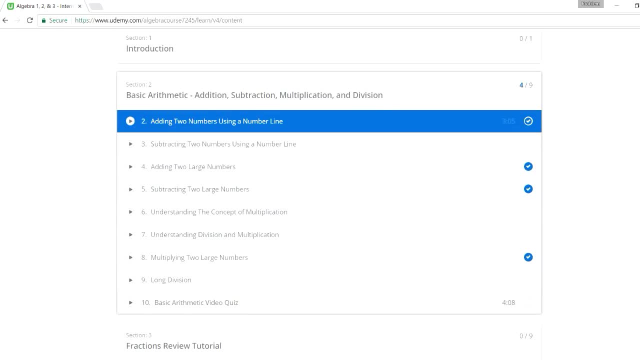 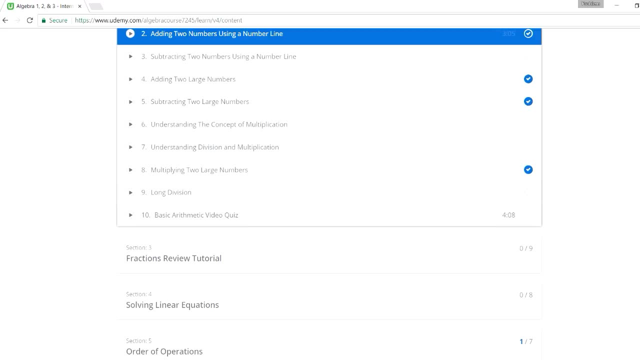 multiplication and division And it has a video quiz at the end. It's a multiple choice video quiz. You can pause it, work on the problems and see the solutions. It covers long division, multiplying two large numbers and things like that. The next: 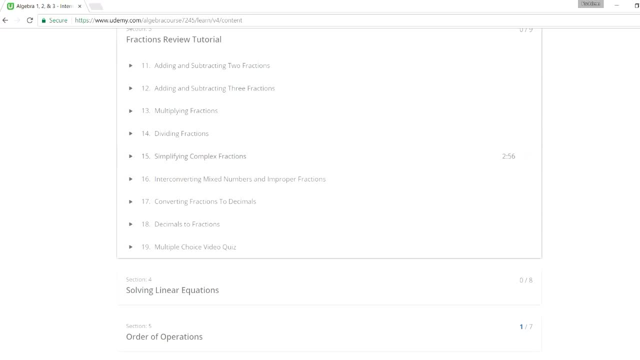 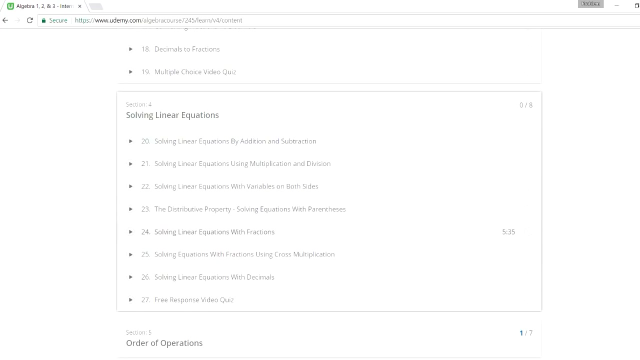 tutorial is on fractions, Add-in, subtracting fractions, multiplying, dividing fractions, converting fractions into decimals and so forth, So you can also take a look at that. Next, solving linear equations, which we covered, And just more examples if you need more help with that. The next topic, order of operations, which 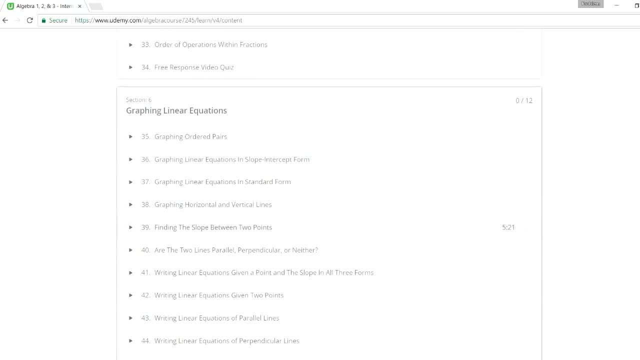 is also useful Graphing linear equations. You need to know how to calculate the slope, You need to be familiar with the slope intercept form, standard form and just how to tell the slope Lines are parallel, perpendicular and so forth. And it's a quiz that goes with. 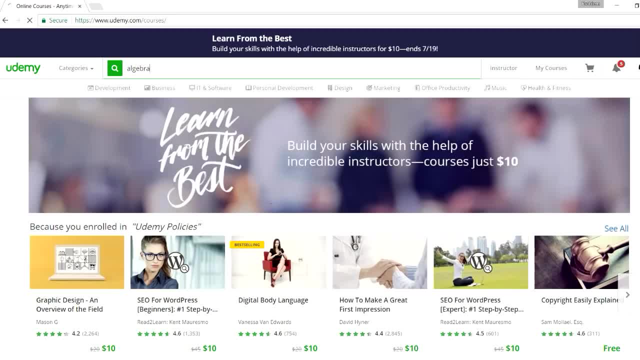 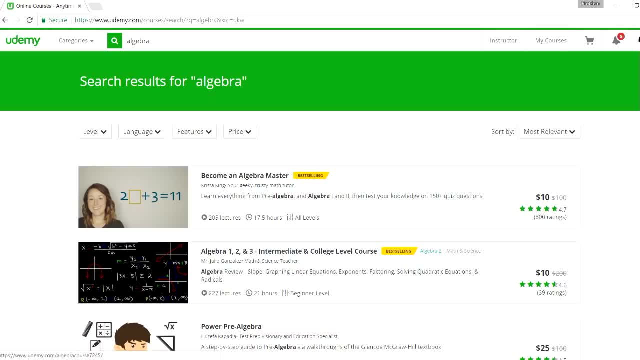 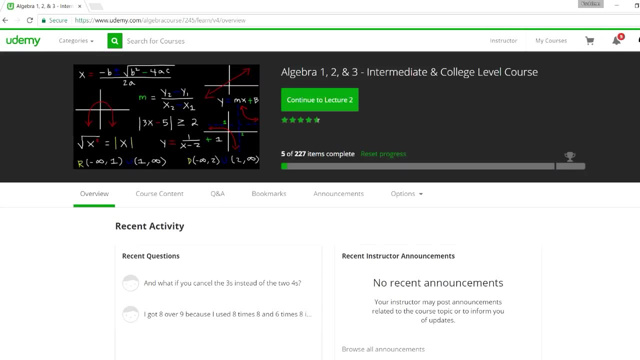 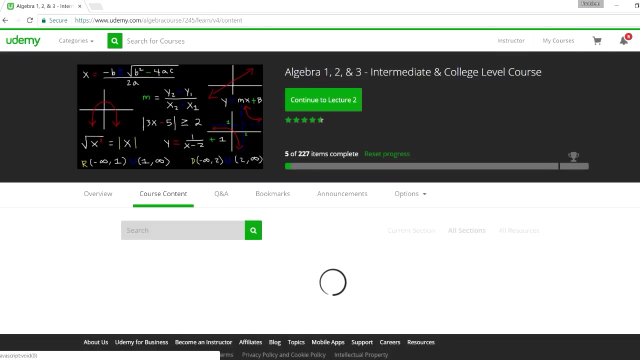 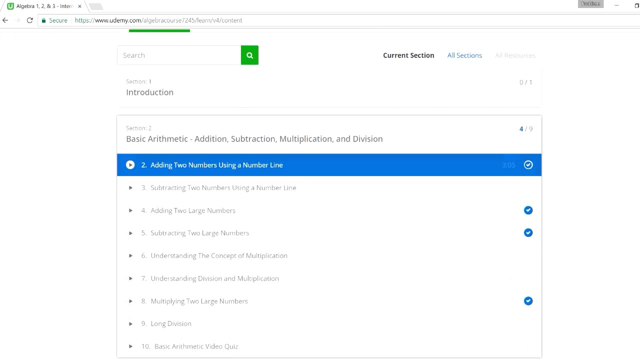 just type in algebra should come up. so it's the one of the image with the black background. so if you select that option and if you decide to go to course content, you can see what's in this particular course. so the first section, basic arithmetic. for those, 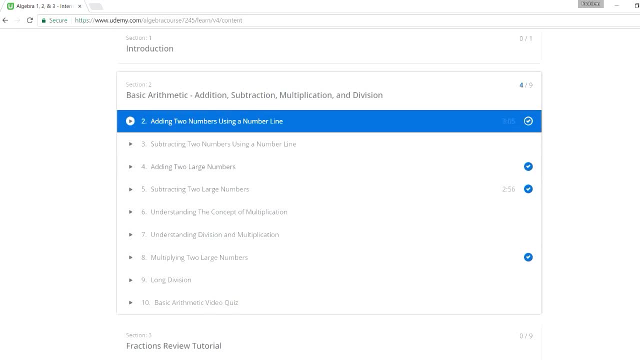 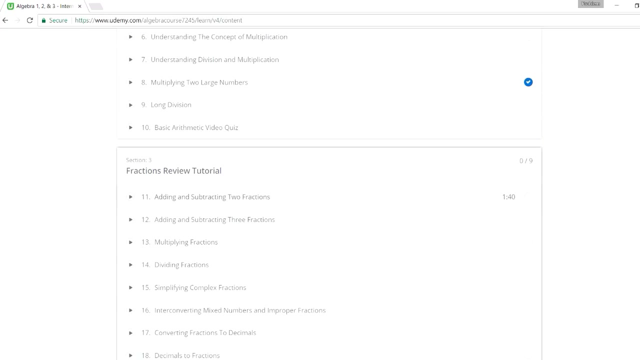 of you who want to focus on addition, subtraction, multiplication and division, and it has a video quiz at the end. it's a multiple choice video quiz. you can pause it, work on the problems and see the solutions. it covers long division, multiplying two large numbers and things like that. the next tutorials on: 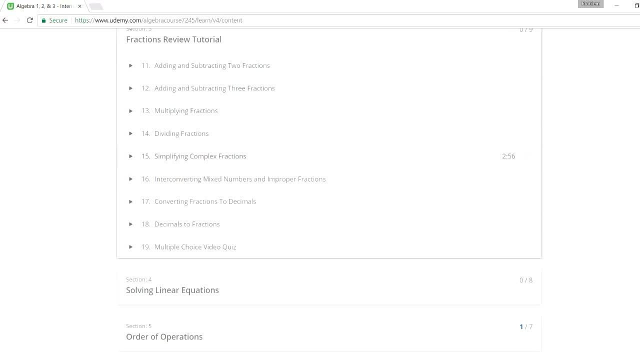 fractions. add in subtracting fractions, multiplying, dividing fractions, converting fractions into decimals and so forth. so you can also take a look at that. next, solve the linear equations which we covered and just more examples if you need more help with that. the next topic: order of operations, which is also useful: graph in linear equations you need to. 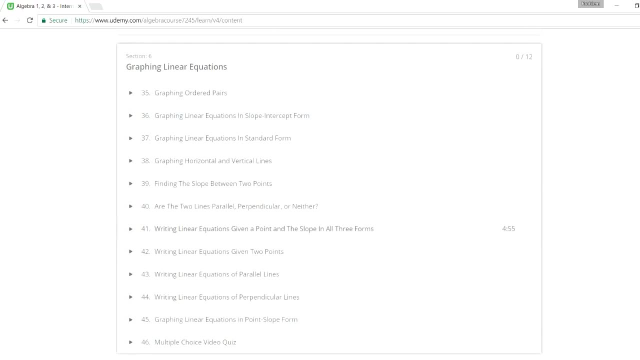 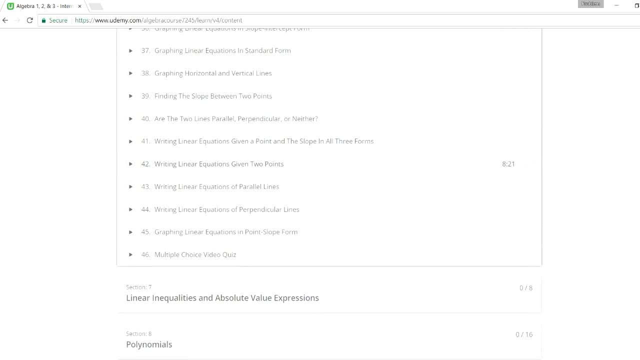 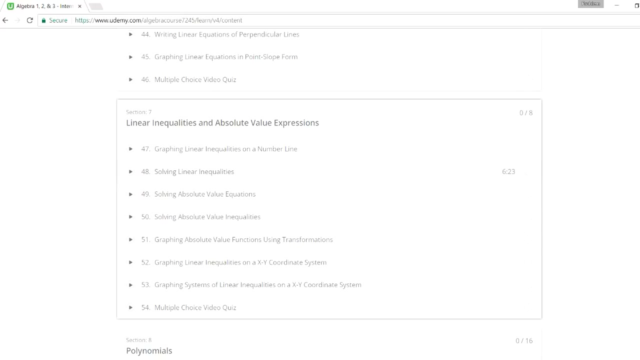 know how to calculate the slope, needs to be familiar with the slope intercept form, standard form and just how to tell if lines are parallel, perpendicular and so forth, and as a quiz, that goes with that as well. the next topic is on inequalities and absolute value expressions, which are also seen- a typical algebra course. and then we have polynomials and 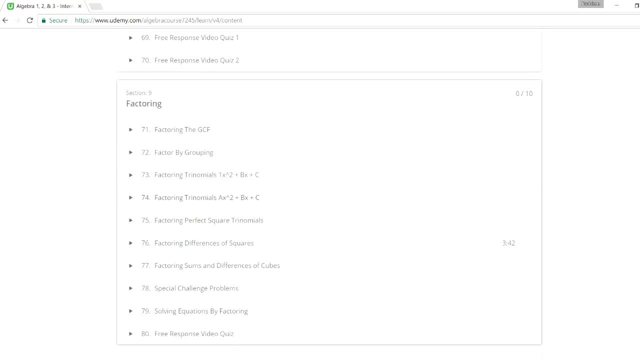 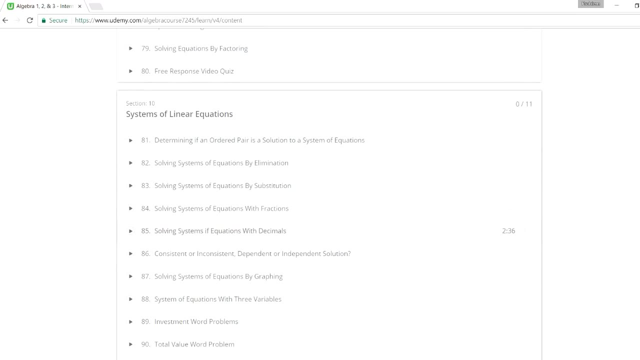 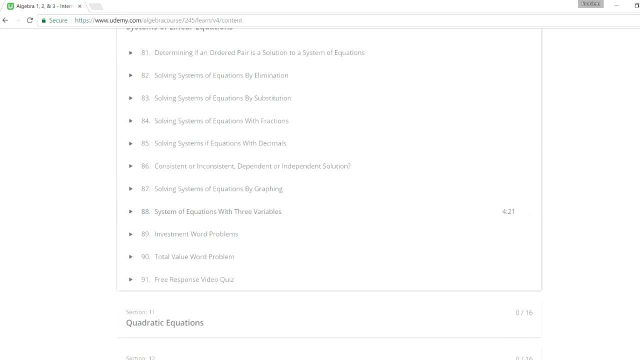 that's a long section, and then factoring you- just that's another topic you need to master. and then system of equations: you can solve it by elimination, substitution. there's also word problems as well. sometimes you got to solve equations with three variables- x, y and z, so that 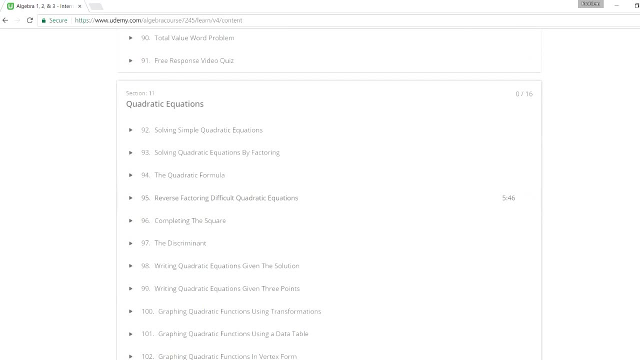 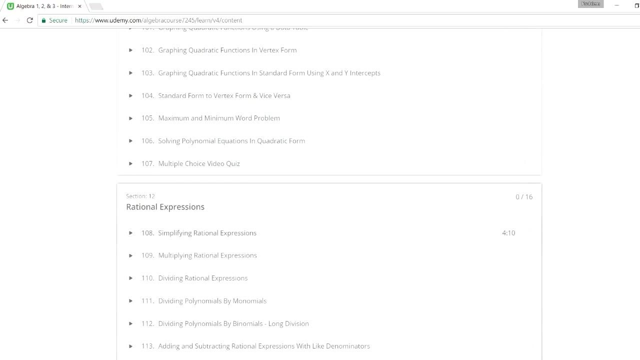 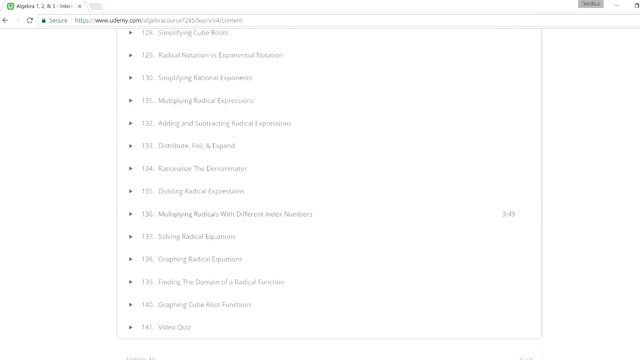 could be helpful. next, quadratic equations: how to use a quadratic formula, how to graph them, how to convert between standard and vertex form, and then you have rational expressions and radical expressions, solving radical equations, simplifying it, things like that, and every section has a quiz so you can.